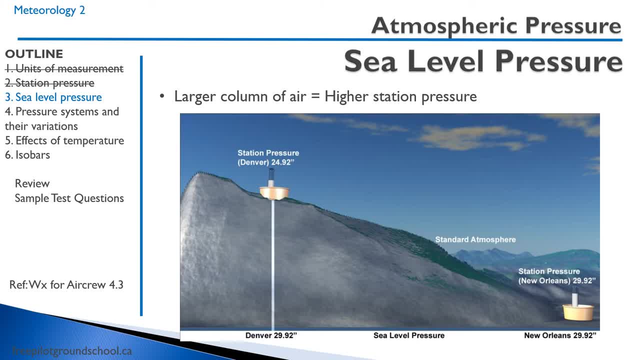 It is the pressure that is at sea level. So, even though the station pressure might be different, we talk about the station pressure at sea level at a given airport. What this allows us to do is get the altimeter setting If we know the station pressure and 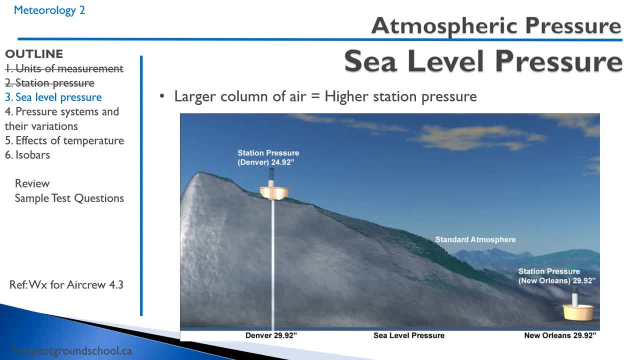 the elevation of an airport, then we can figure out what the sea level pressure is. Once we know the sea level pressure, that is the altimeter setting, then air traffic control can give every aircraft the altimeter setting and then that makes sure that everybody, all the aircraft, 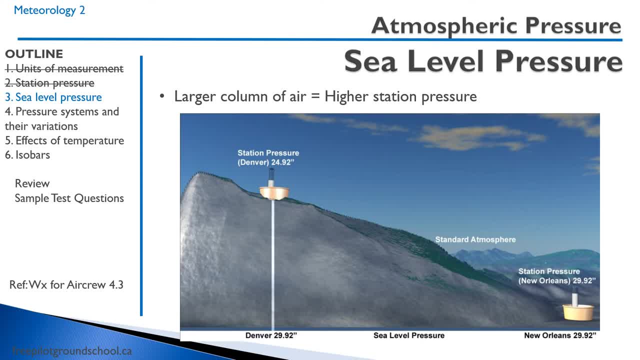 same altimeter setting and the same altitude, or at least there is some sort of a standard. So a higher column of air means a higher station pressure. So at sea level there will be a higher column of air above it. so the pressure is going to be higher at sea level than it will be at the 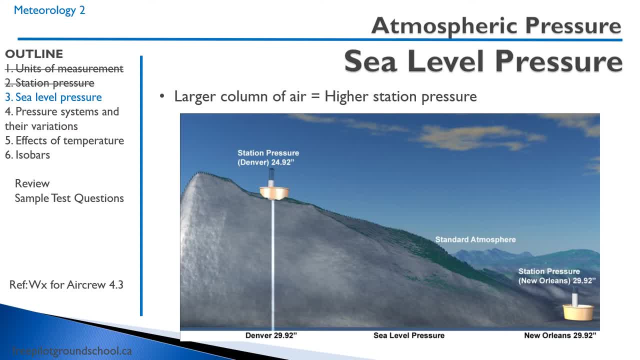 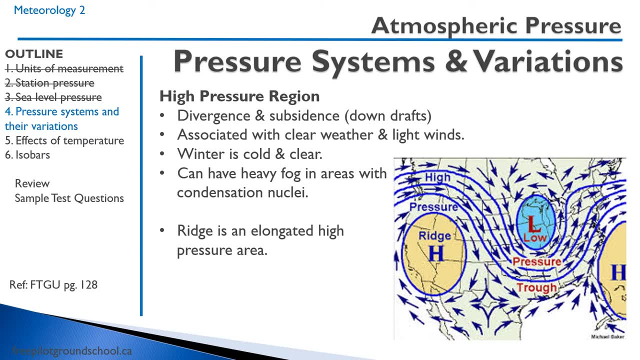 station pressure, which may be higher. So here we start talking about atmospheric phenomenon. So we're going to discuss in the next couple slides pressure systems and variation. So first off, let's talk about a high pressure region. if you look here, the big h indicates. 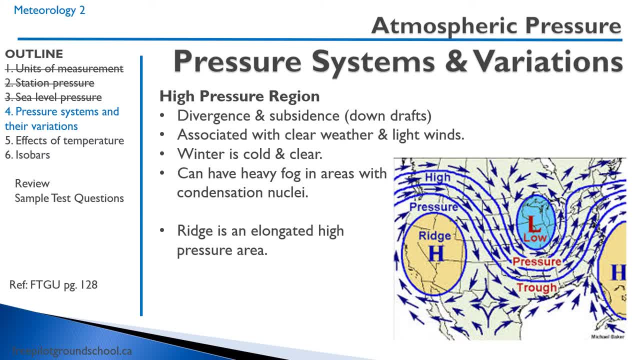 a high pressure region. it's obviously an area where the atmospheric pressure is relatively higher than area, than the surrounding areas. High pressure regions are generally associated with divergence and subsidence, so that's downdrafts. So if you think about it- the high pressure region, the air will want to go outwards from the high pressure region. 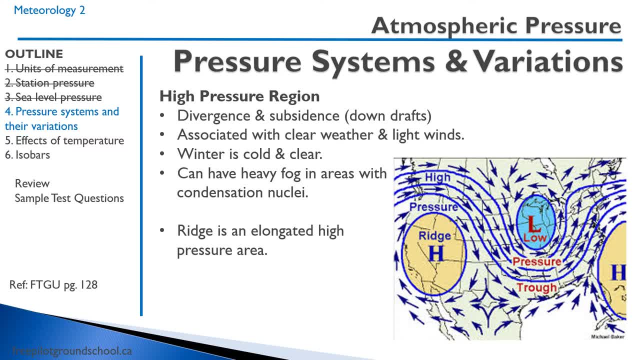 let's say, divergence, and that air has to be replaced somewhere, and it's replaced from the air above it. so that's why you have the sensitive. the boundary high pressure regions are typically associated with clear weather and light winds. in the winter time, this means cold and clear air. 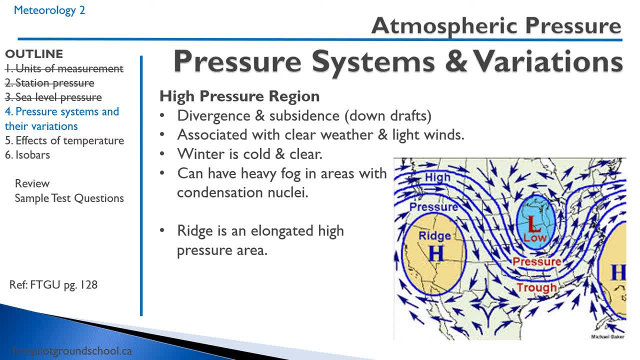 often for days at a time, it's kind of a beautiful cold winter day. that's a high pressure region. however, in some areas, uh with uh an abundance of condensation nuclei- i will learn more about that later- you can end up with very, very heavy fog, probably the heaviest fog i've ever seen. 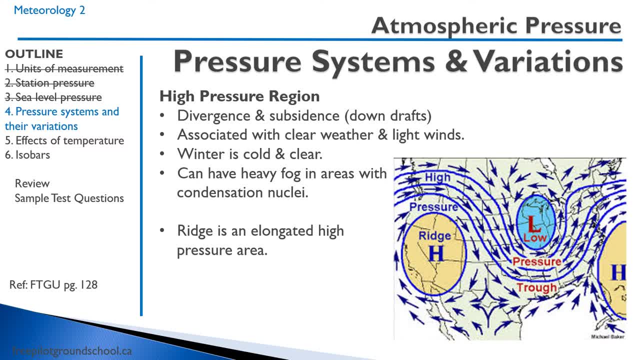 in my career was in a for a couple days was actually in a town called prince george, british columbia. there's a number of pulp notes there. there's a high pressure system there and because the pulp mills had a lot of smoke, condensation nuclei and all the moisture 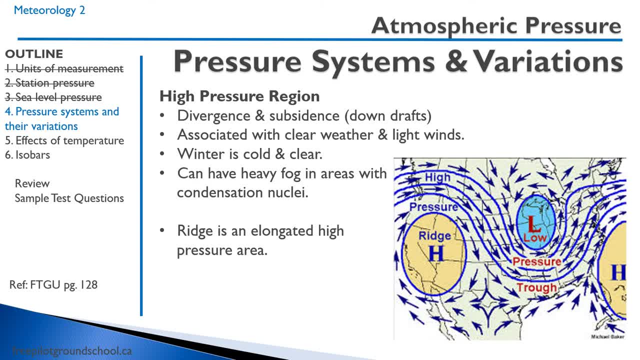 just got pushed right down onto the town and onto the airport, uh, for for several days could also have a rear ridge is an elongated high pressure area. so you look at the uh image: on the right we have the high pressure and then here we have a ridge and you can kind of see it makes. 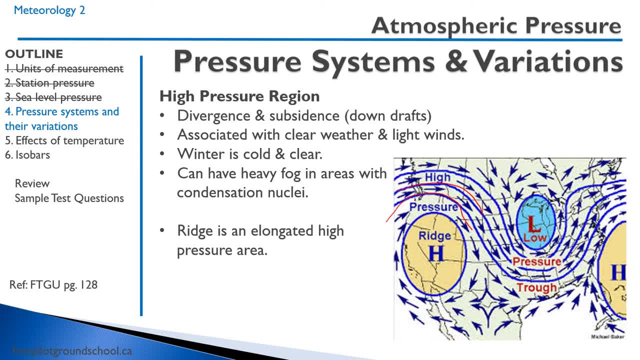 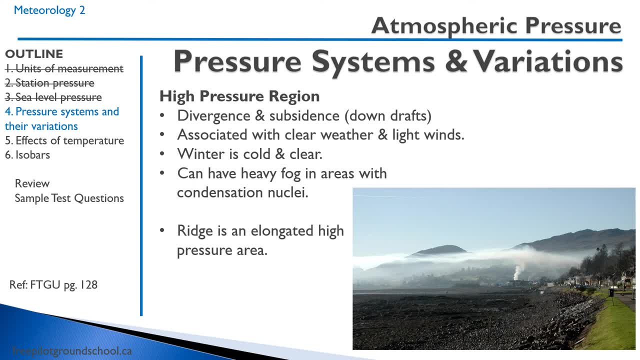 makes this ridge uh thing. it's an example of how high pressure can produce condensation nuclei here, of what i mentioned, how you can end up with fog. you can see it's a beautiful, clear day. however, the smoke coming out from whatever this industrial site is presents condensation nuclei and it's getting forced down by that. 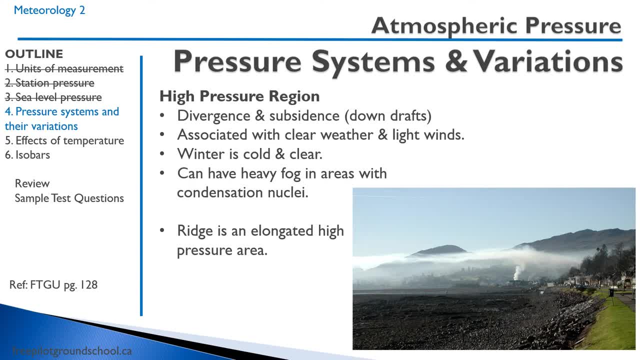 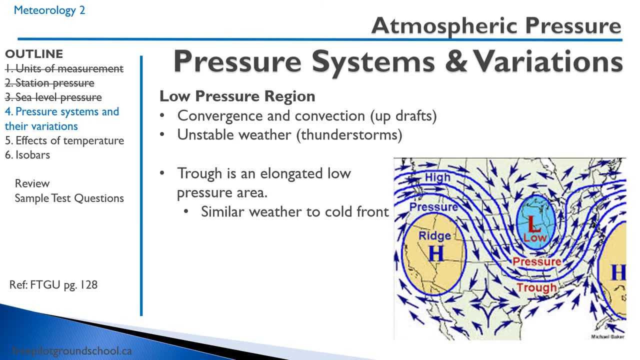 high pressure region, leaving a layer of smoke or haze over the area. university, we can have a low pressure region and a low pressure region. you can imagine that the air comes from the surrounding areas and goes into the low pressure in the middle. So what that means is you have convergence and convection, You have updrafts. 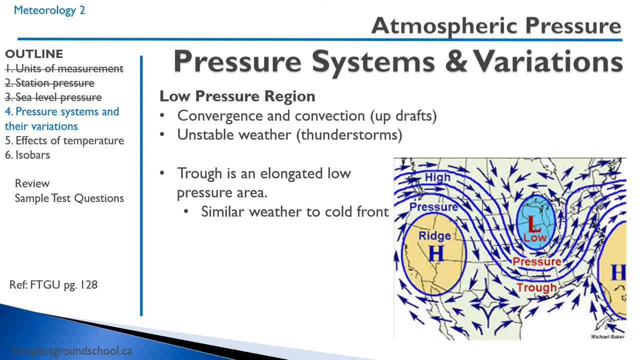 The air comes from surrounding areas into the low has nowhere to go but up, And so often we end up with unstable weather such as thunderstorms. because the air is converging and then there are updrafts, We can have a modification of a low pressure region. that's called a trough, So it. 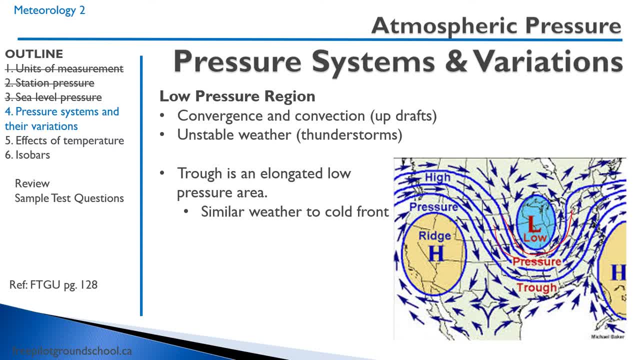 looks just like- well, like- a feeding trough right here. Okay, And this is kind of an elongated low pressure area. Weather at troughs is similar to cold fronts. We'll learn about that later. You can end up with strong winds and unstable, miserable weather. 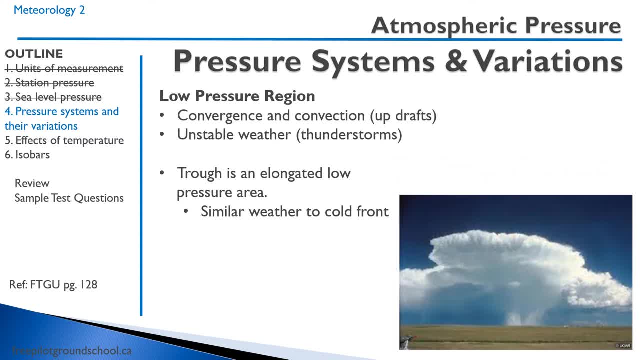 The picture of unstable air from a low pressure region. Here's that massive cumulonimbus mummatus cloud And you can just imagine that you're going to end up with very unstable air, high turbulence, thunderstorms, hail, that sort of thing in a strong low pressure region. 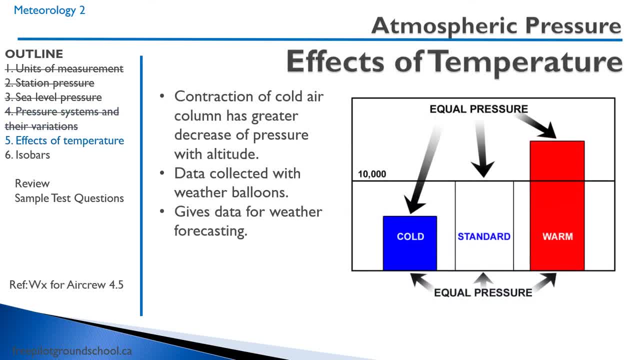 Temperature can affect atmospheric pressure. So the contraction of cold air, of a cold air column, has a greater decrease of pressure with altitude. because it's more dense, Everything kind of sits lower And conversely, warm air will have a greater change of pressure with that altitude. These data are collected using 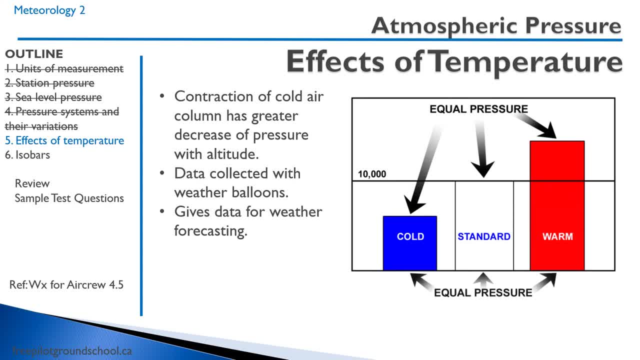 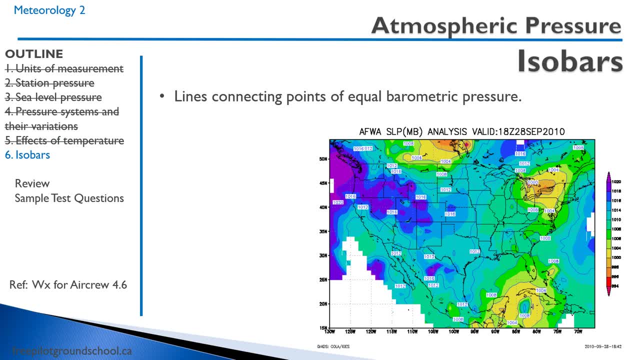 weather balloons and are very important for weather forecasting. Iso bars are lines connecting points of equal barometric pressure. You'll see isobars on weather maps, surface analysis maps and forecast maps as well. Here they are kind of a blue color, So let's. 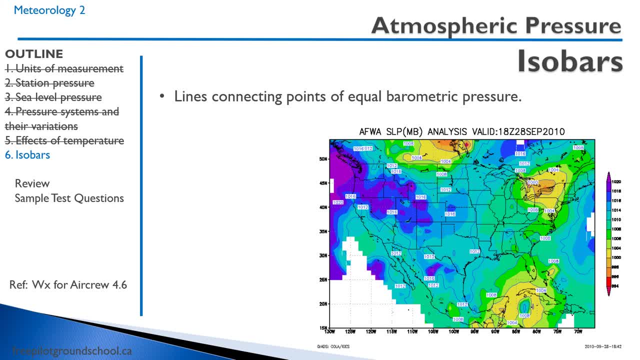 just take a look at them. here I just have a red pen And so you can see this line right here. I'm just drawing it right following it. Okay, that right there has a pressure of 1,016, or looks like 1,012, hectopascals. So if you just 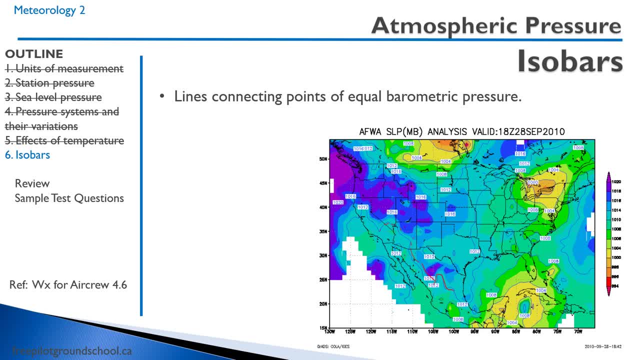 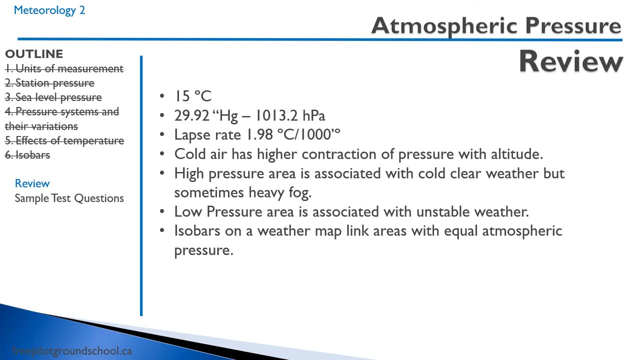 follow this around. we'll make like a ring and you can kind of think of it as similar to contour lines on a topographic map. This is kind of what the pressure is like. Remember we use standard atmosphere. the units 15 degrees Celsius, The atmospheric pressure 29.92. 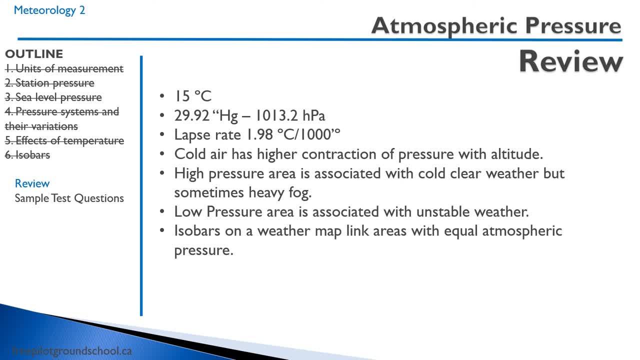 inches of mercury, or 1,013.2 hectopascals, and a lapse rate of 1.98 degrees Celsius per thousand feet. Cold air has higher contraction of pressure with altitude than warm air. High pressure area is associated with cold, clear weather, but from 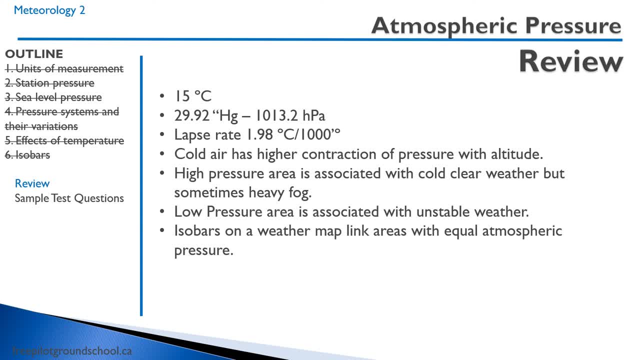 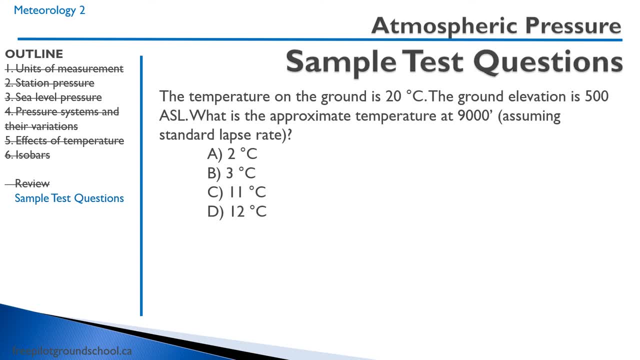 low jump heures. sometimes heavy fog, low pressure, areas associated with unstable weather. Isobar on the weather map link areas with equal atmospheric pressure. Okay, here's our first sample test question. The temperature on the ground is 20 degrees Celsius. The ground elevation is 500 feet ASL. What is the approximate temperature at 9000 feet? 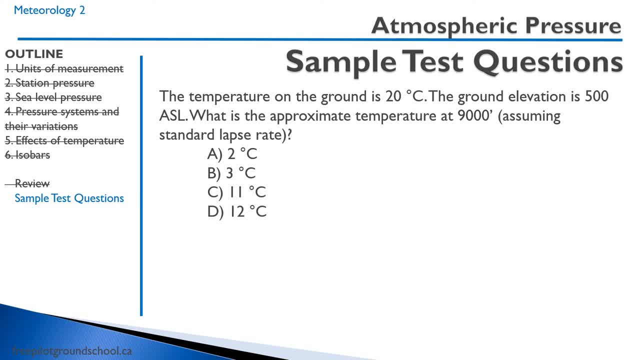 assuming a standard lapse rate- 地溶口- So gridlines- 500 feet, So 9000 feet minus be 8,500 feet approximately. If we recall, our standard lapse rate is approximately two degrees per thousand feet, So we have eight and a half thousand feet multiplied by two. So that would be. 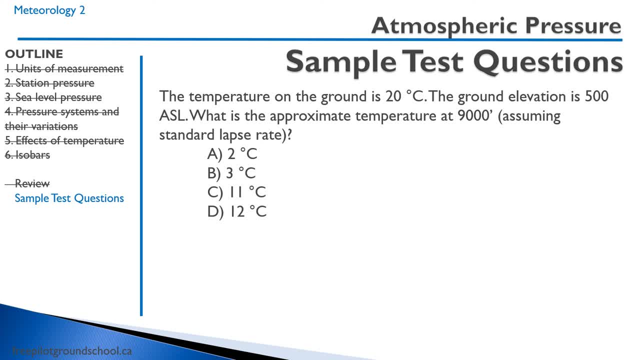 17. So 20 minus 17.. Maybe I'll just actually draw this out or write this out: 9,000 feet minus 500.. Just make it clear: Equals 8,500 feet times two degrees Celsius per thousand feet. 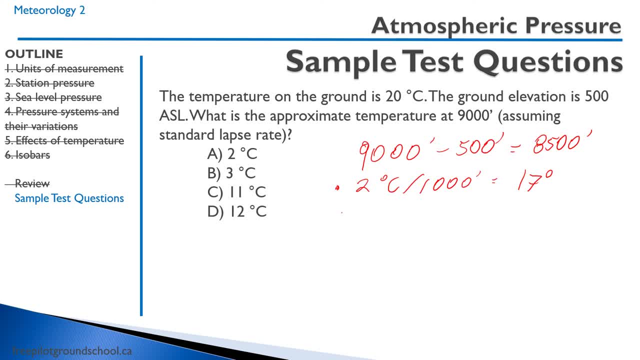 So that's going to be 17 degrees. So we start at 20 degrees minus 17 degrees equals three degrees C. So the correct answer is going to be B, three degrees. What type of weather can be expected at low pressure system? So remember low pressure system. 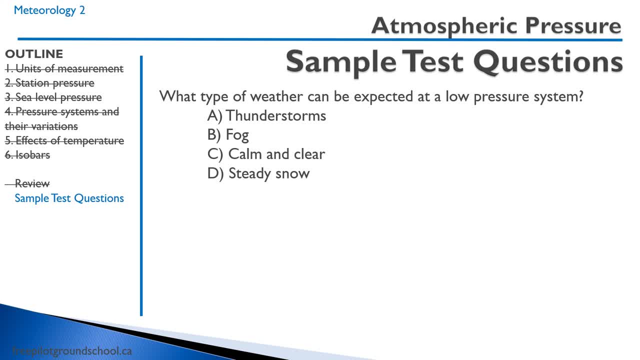 has convergence and updrafts unstable air. So A thunderstorms, Yeah, you're going to see thunderstorms. B fog- No, not usually. Fog is when the air is very stable, Calm and clear. It's usually high pressure system, so that's not correct. And steady snow. 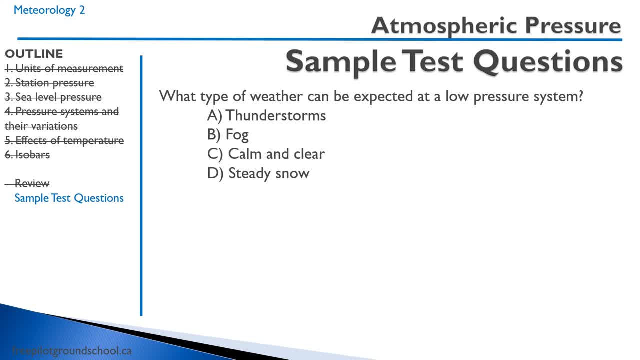 No, not usually steady snow. So the correct answer: A thunderstorm. What type of weather can be expected? A high pressure system in the winter, So remember you're going to have very stable air. So A thunderstorms, We can rule that out. B fog: Generally not, It's rare, It is possible. 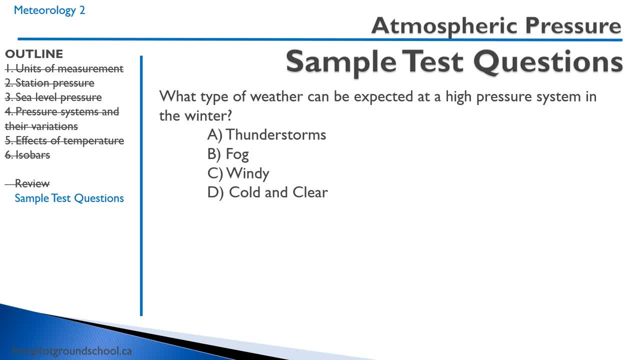 but it's great weather: C, windy. No, that's usually associated with trough D, cold and clear, So that's the correct answer. Thanks all for joining me. We'll see you on our next meteorology lesson.